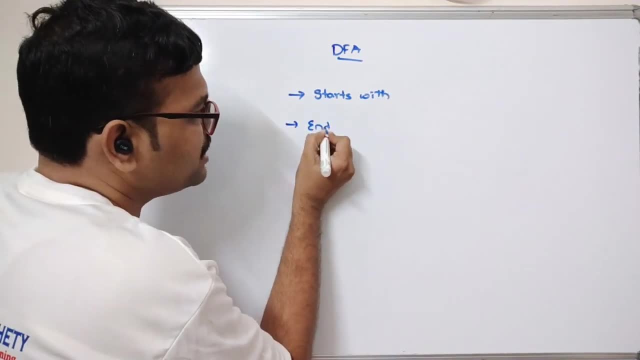 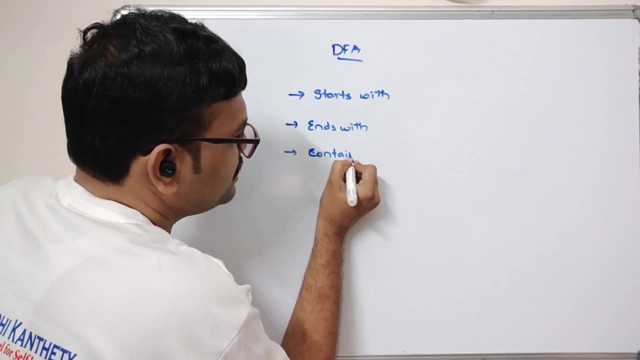 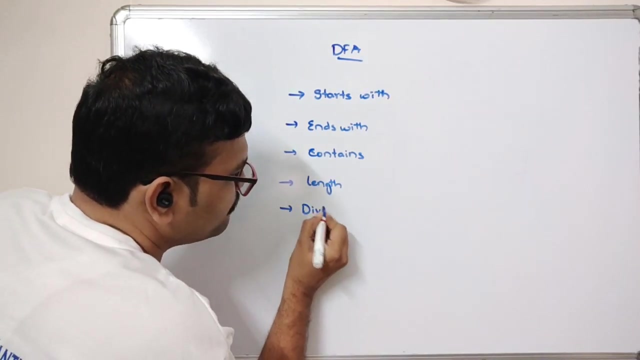 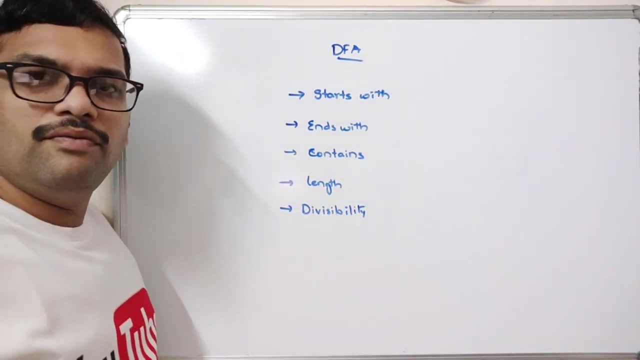 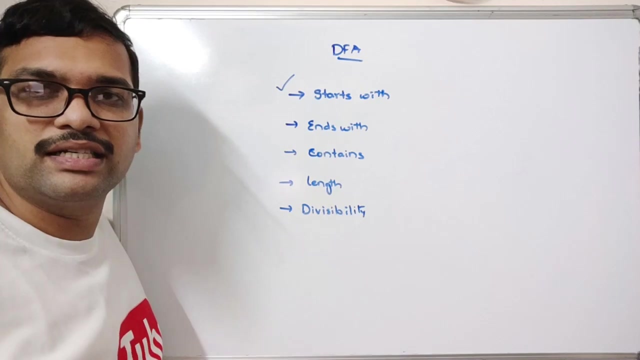 substring And similarly. the next one is ends with and next contains: And length problems, length of a string- and divisibility problems, divisibility problems. So here we will start with this one starts with, and further sessions will go with, ends with: contain length and divisibility. So how can we construct the DFA? Now let us start. 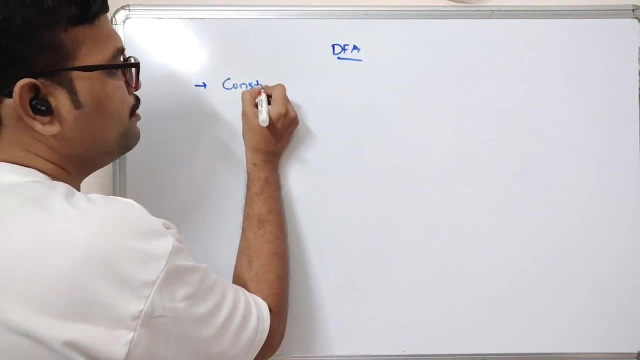 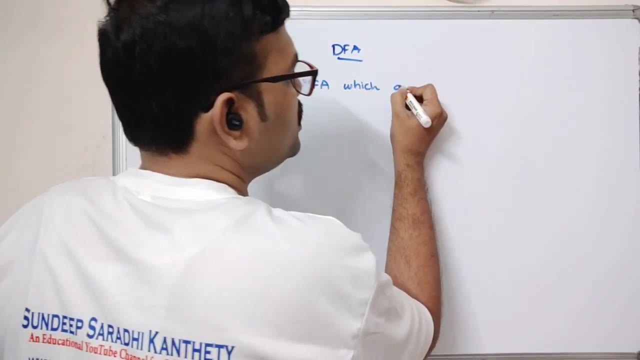 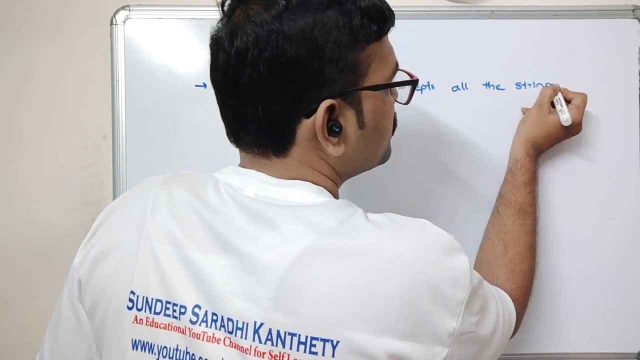 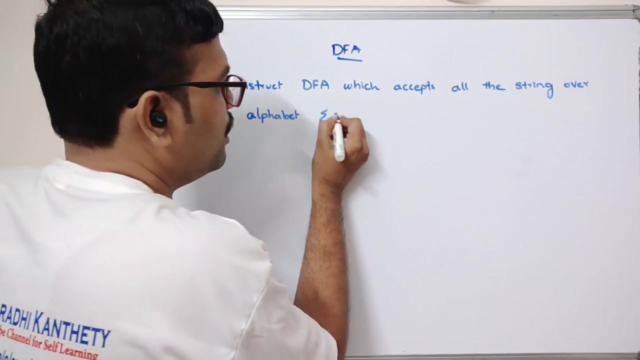 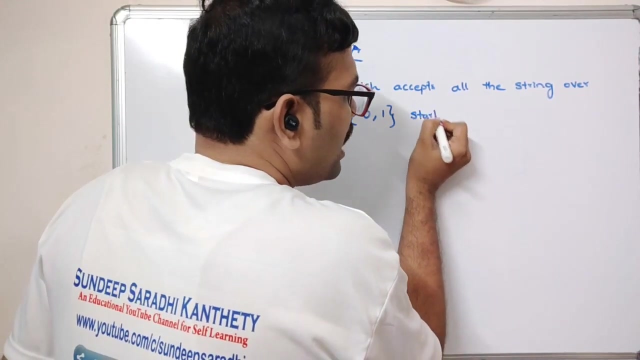 here. So construct DFA. A question will be: construct DFA. DFA which accepts, which accepts all the strings, all the strings over alphabet sigma is equal to zero, one, zero. one Starts with, starts with starts with zero, the strings zero. 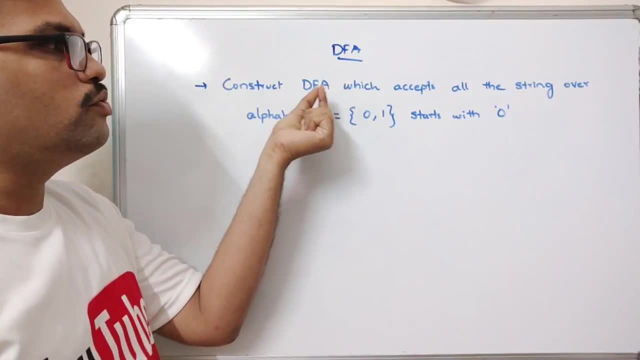 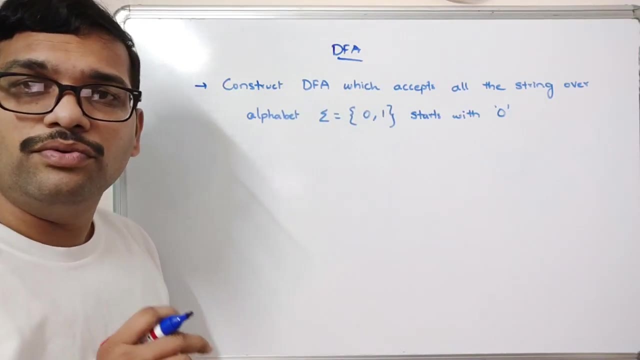 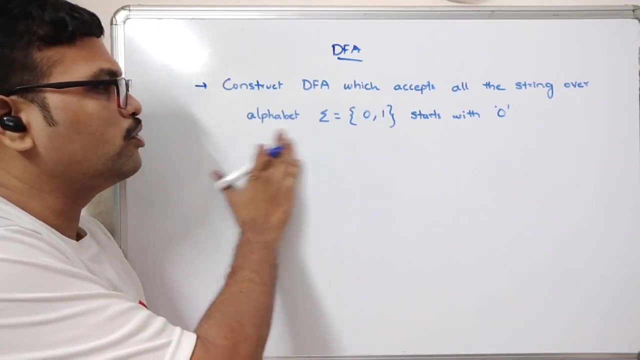 So here the question is: we have to construct the DFA so which accepts all these strings over the alphabet. 01 starts to zero. So first thing is we have to write the language. So here the language is a collection of strings. So we have seen all these things About this alphabet, about this string, about the language. 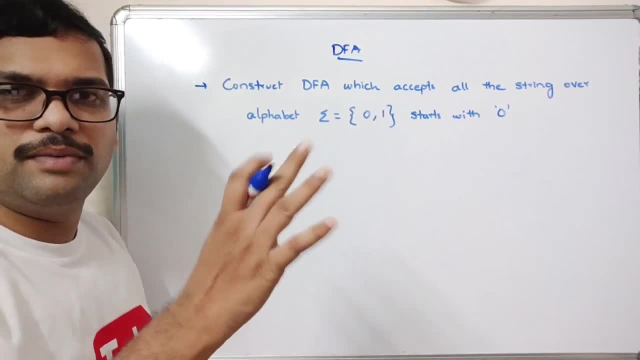 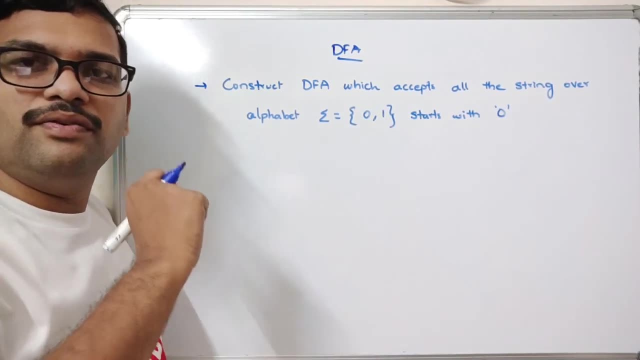 We have seen in the previous session about what joined the string r Kotan and read the previous sessions, so i will post the previous session links in the description so that you can follow that. so first of all we need to write the language which satisfies this condition. that means: 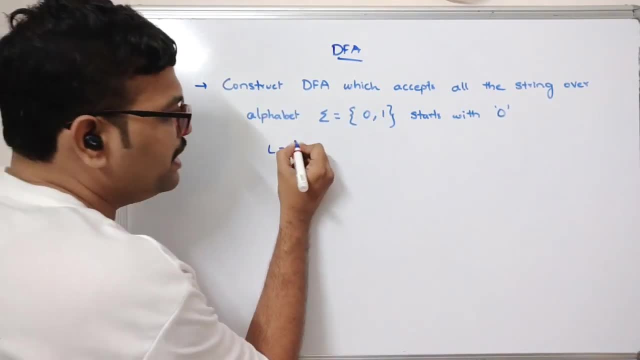 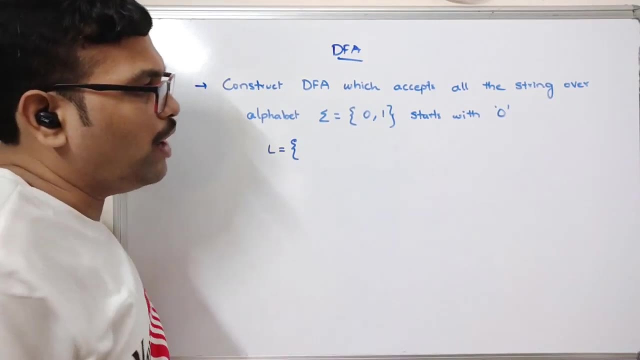 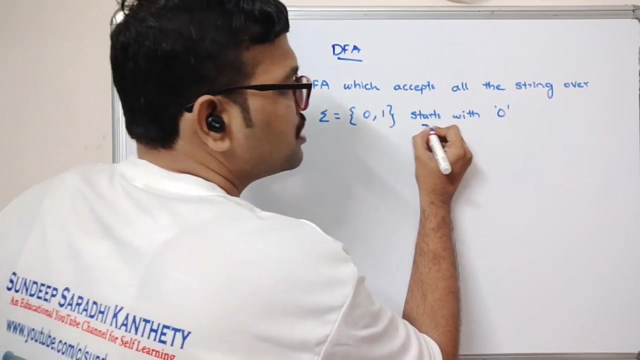 starts with 0. so let us represent language as l. l is equal to here. the string is the collection of symbols over the alphabet 0 and 1. so we need to prepare the 0 and 1- i mean the strings- with the 0 and 1. so first it should starts with 0. the condition is it should starts with 0, so the 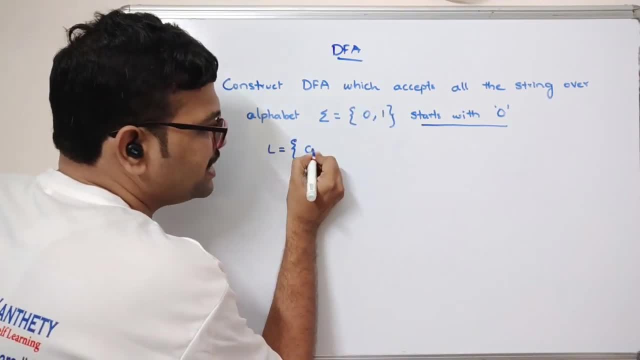 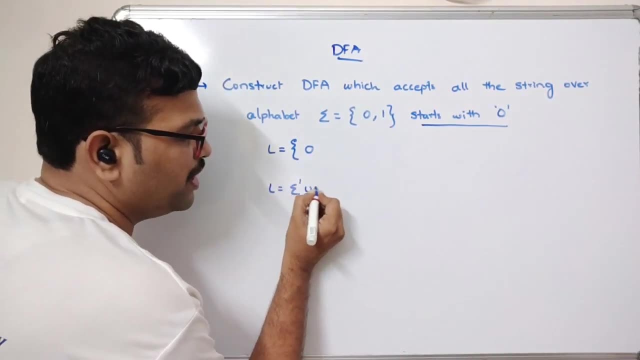 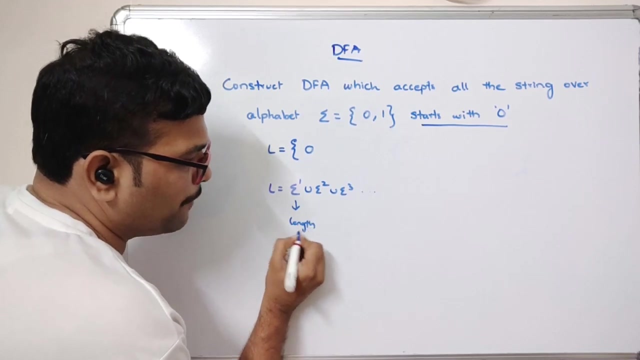 minimum. you just write from the minimum. so minimum means the single digit. okay, so we know that l it can be written as sigma 1, union, sigma 2, union sigma 3, etc. etc. so 1 mean length, 1, sigma 2 means length 2, sigma 3 means length. 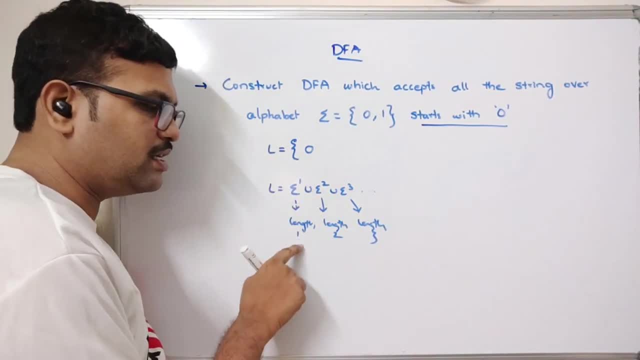 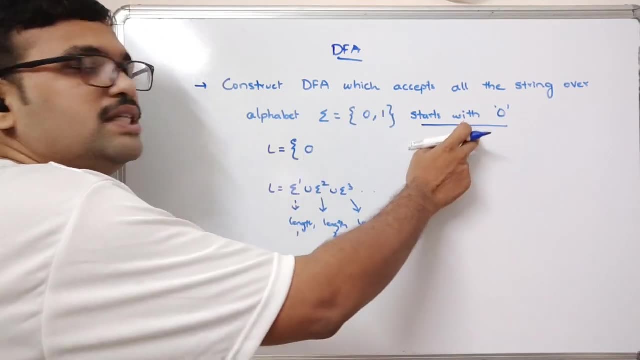 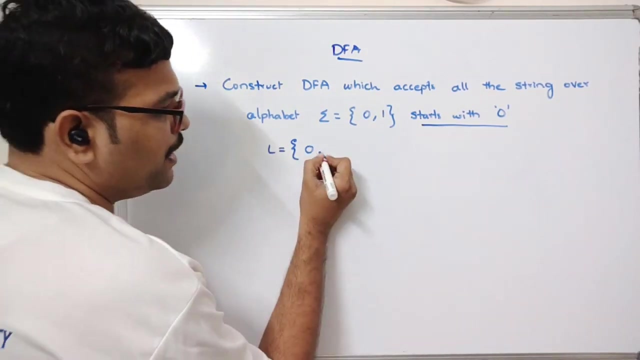 3. so just write down the strings of length 1 first and then go to the length 2, then go to the length 3, and just remember we have to write the strings which satisfy this condition, but that means the string should start with 0, only so coming to the length 1 0 itself and coming to the next second. 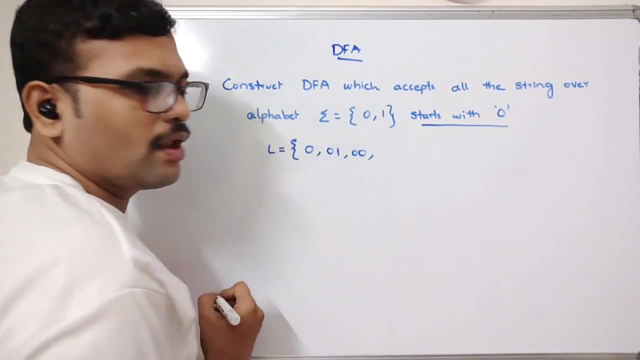 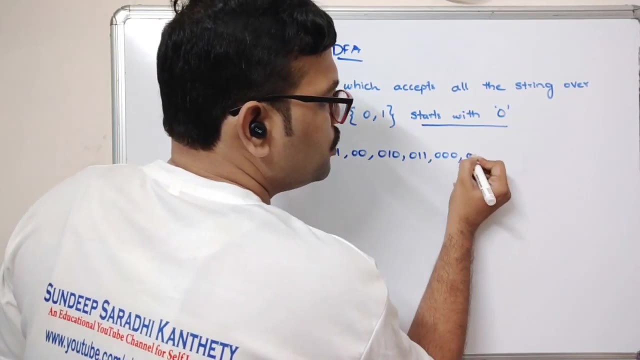 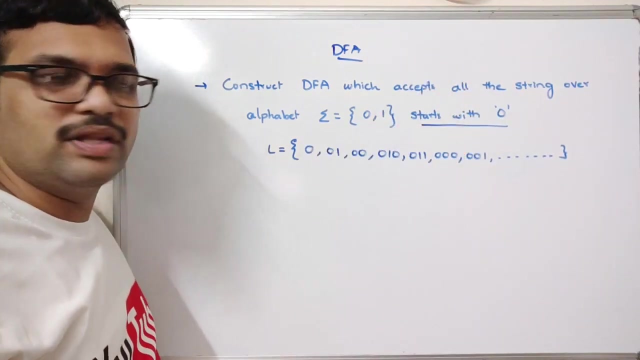 level. let us take 0, 1, 0, 0. okay, next category: 0, 1, 0, 0, 1, 1, 0, 0, 0, 0, 0, 1 and so on. we get more number of strings, so with a multiple lengths. so that's why this. 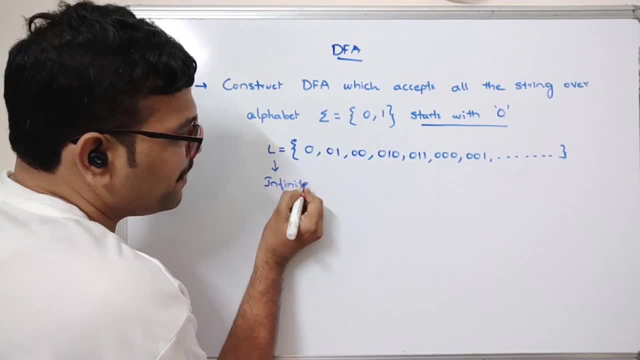 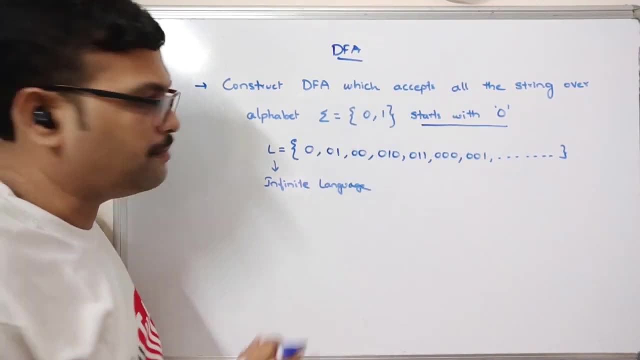 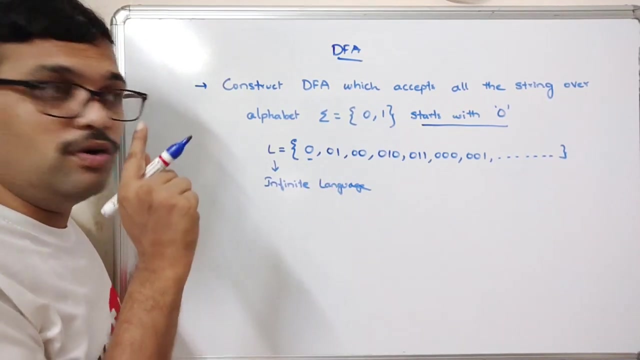 language is an infinite language. this language is an infinite language, so there is no finite strings. okay, so any string which starts with 0, that's the only condition. so for this, just remember what is the minimum element: 0. so what is the length of this one? 1. so if you want to represent the 1 length, 1 string. 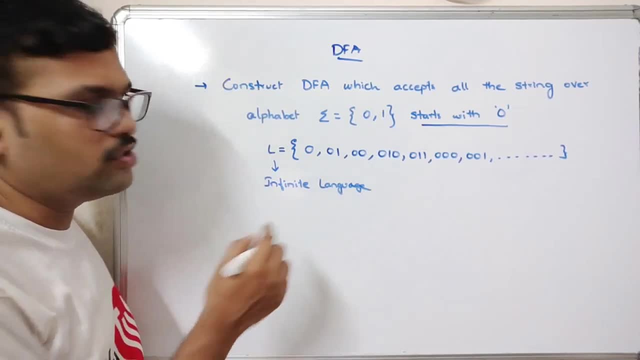 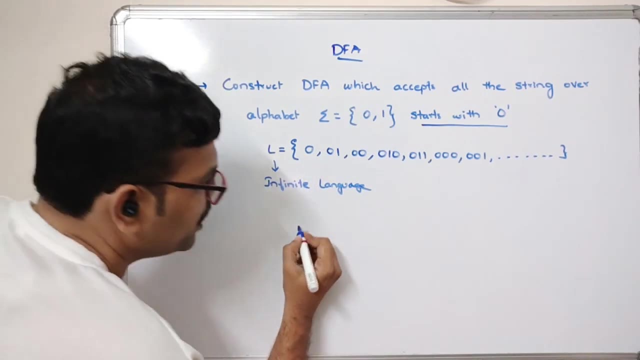 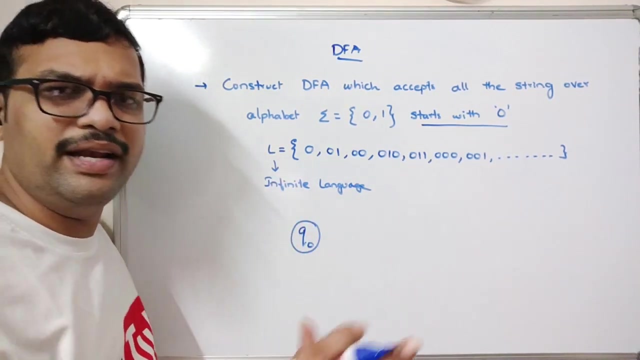 we have to go with the n plus 1 states. so if length is n, n plus 1 states are required to accept this string. so here only one is there. so we require two states. so just i will represent q naught as a state. so you can give any label. so you can give a, b, c, d or any anything else. 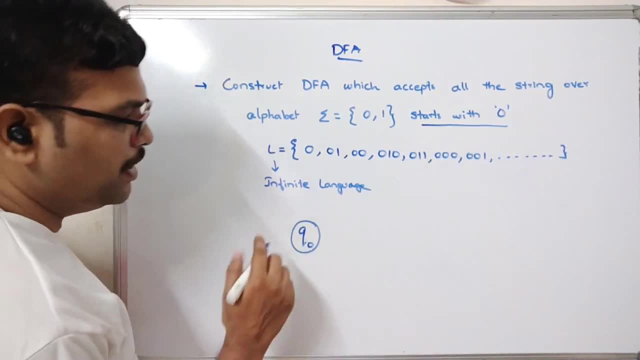 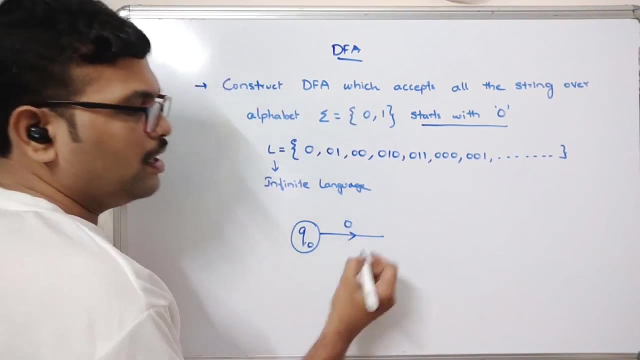 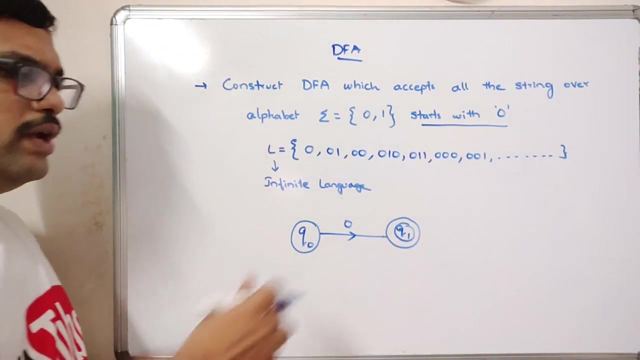 i'll give q naught, q naught, q 1, q 2, q 3 and so on. so q naught is a one label, so q naught. on input symbol 0, q 1, and it should end here, because so it may not end, so it should start with 0. okay, so this is the. 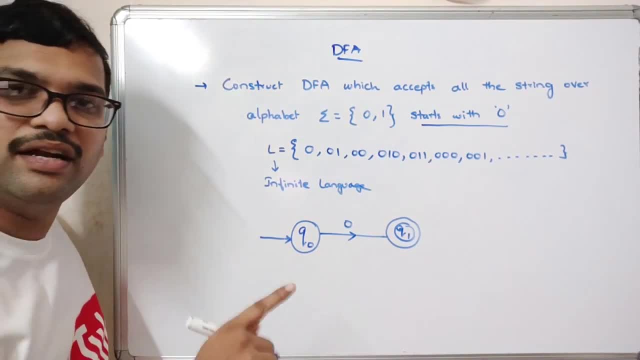 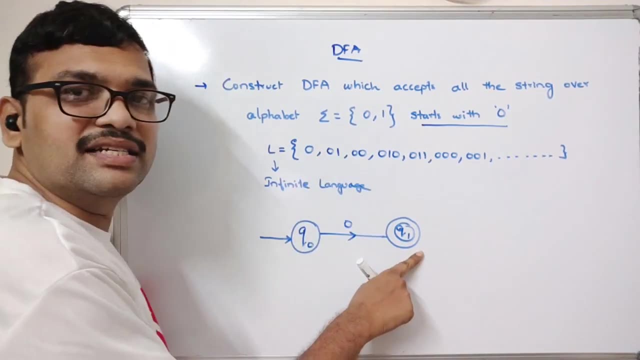 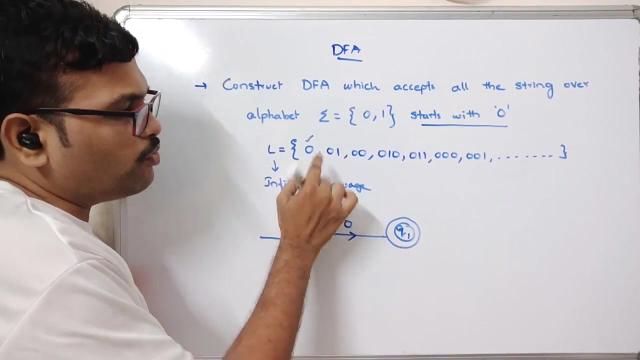 initial state. so this also we have discussed in the previous session. the initial state will be having the edge from no source. so this is the initial state and upon 0 it ends. so this string is accepted. now you can observe here 0. so upon 0 it came. so what about the 1? so 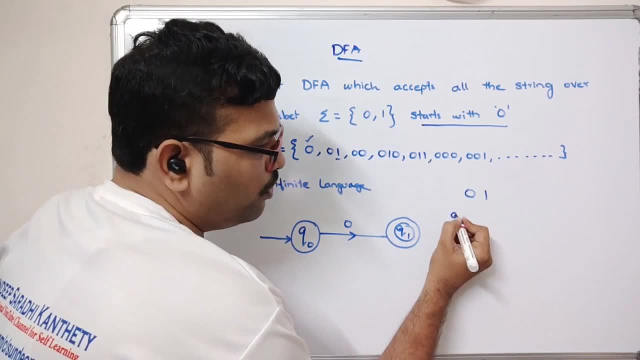 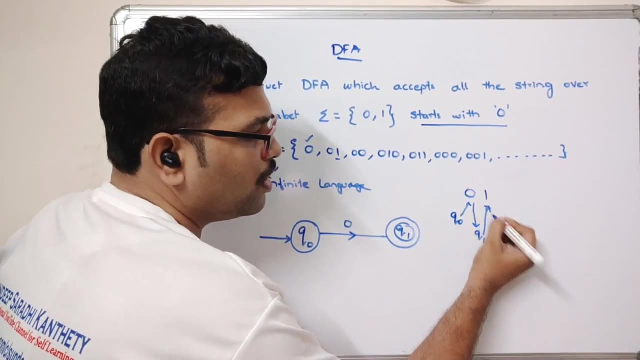 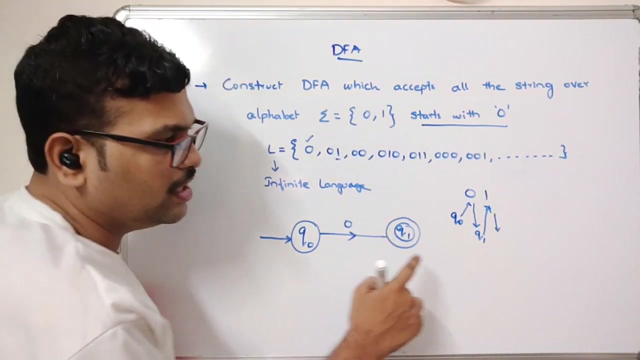 if you are using this 0 and 1, so q naught on 0- it will move to the state q1. and what happens if you, i mean if, if q1 with the input symbol 1, where it should end? so here q1 itself is the end state. so 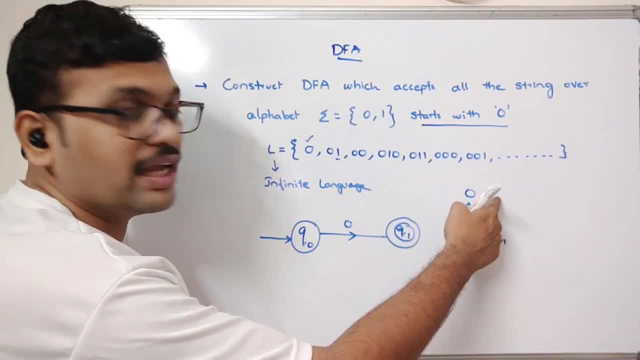 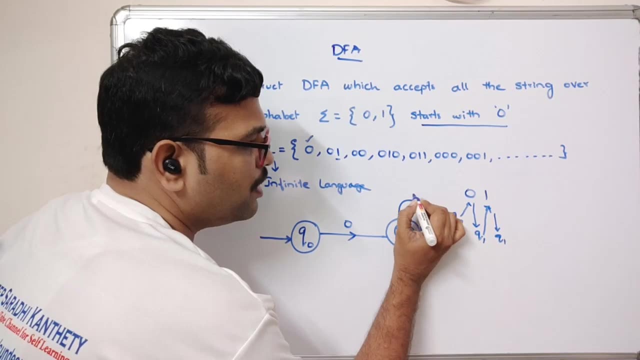 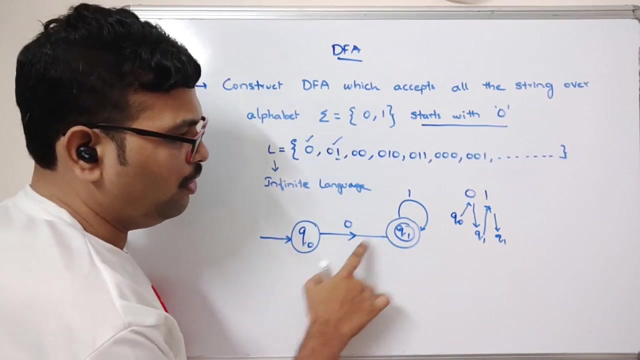 simply you can end here itself, because this is the end end of the string. so simply you can give a self loop a self loop, and whenever it becomes one will remind in the same state. and so this, this is satisfied: 0, 1. now 0, 0. what? 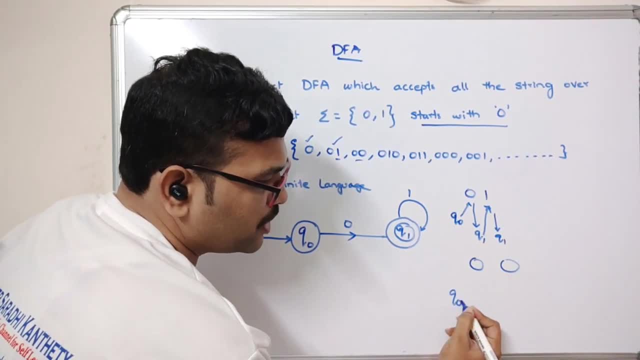 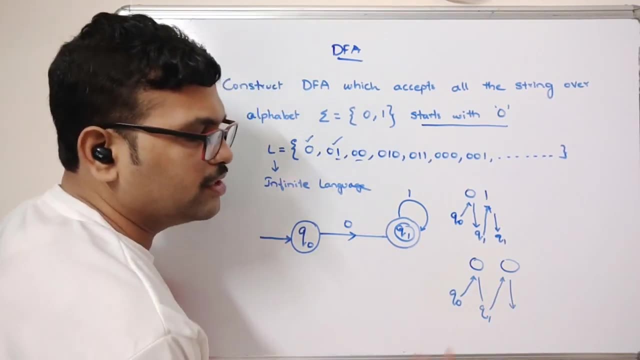 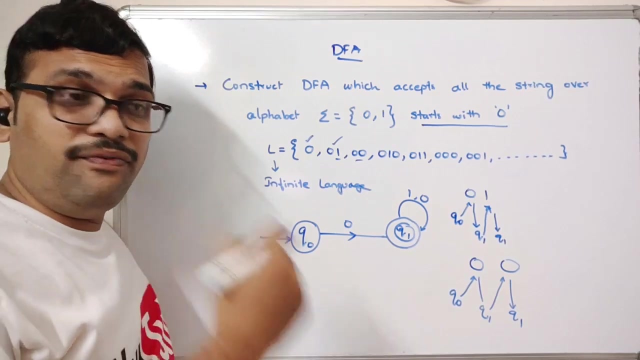 happens. so if it is 0- 0, if you are starting with Q naught, Q naught on 0, it goes to Q 1 again. if Q 1 with a 0, where it should end, so Q 1 is the final state, so here itself it should end. so just use another input symbol. so if Q 1 with 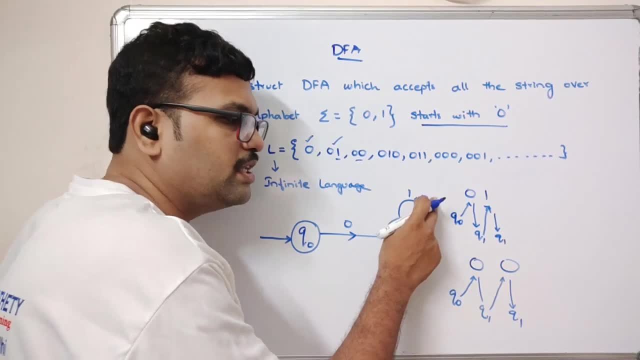 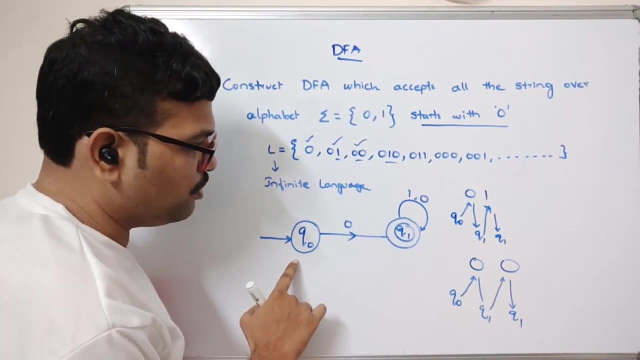 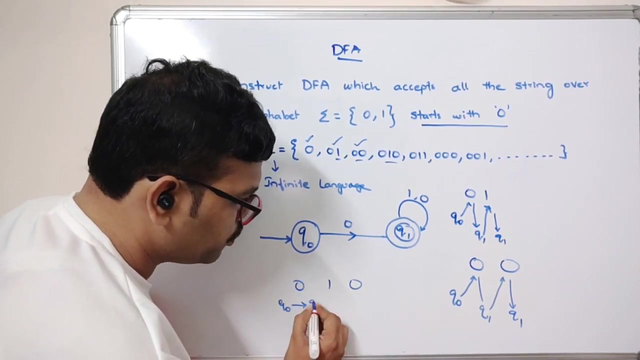 input symbol 1, it remains in the same state. Q 1 with input symbol 0, it remains in the same state. so here you can observe. this was accepted. and coming to the next one: 0, 1, 0. so 0, 1, 0, 0, 1 0. so Q naught on 0, it moves to Q 1. Q 1 on 1 it. 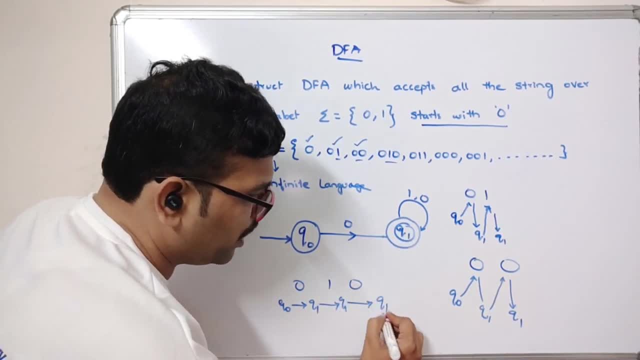 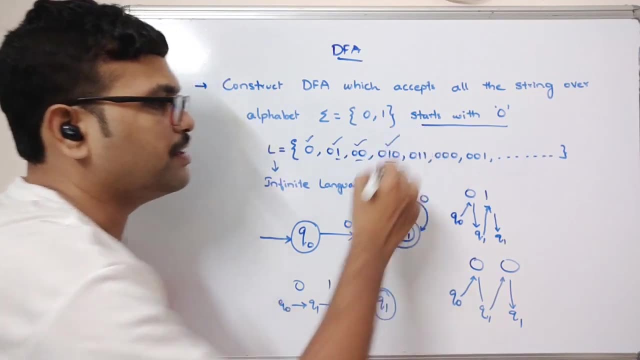 moves to Q 1. Q 1 on 0, it moves to Q 1 and it ends the string right. so what is the final state? Q 1. here also, Q 1 is a final state, so this string is also accepted. so we have to write down the language which accepts all the. 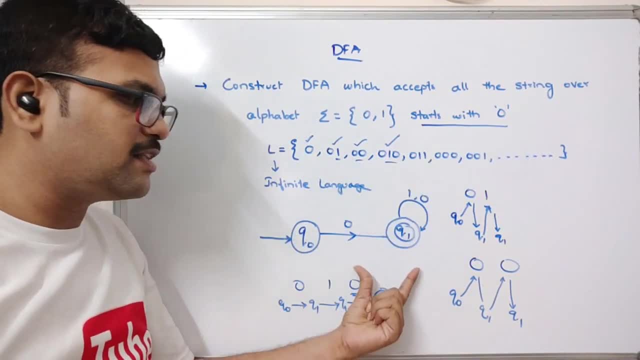 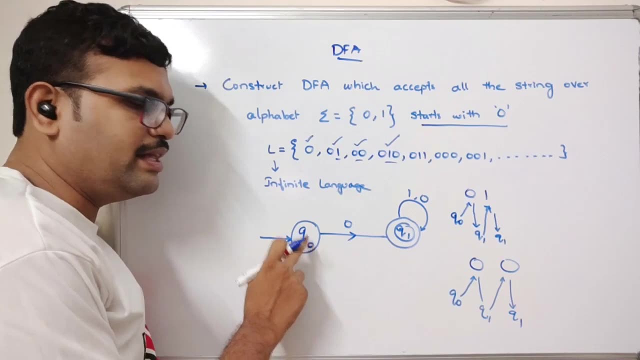 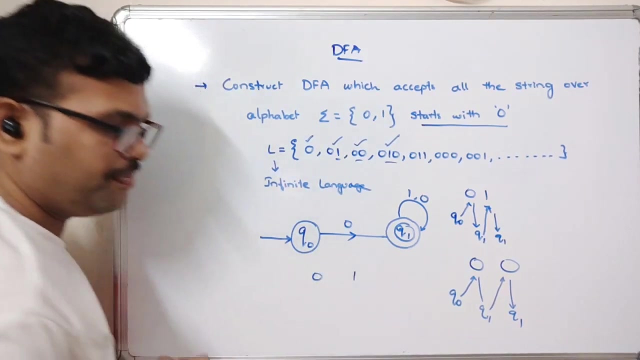 strings which starts with 0, and from this we have to construct the DFA. so we know that DFA means for every state. there should be a transition for every input symbol, for example here you can see this example. so inputs are 0 and 1. inputs are 0 and 1. I will write here itself. okay, so here is the input: 0 and 1. 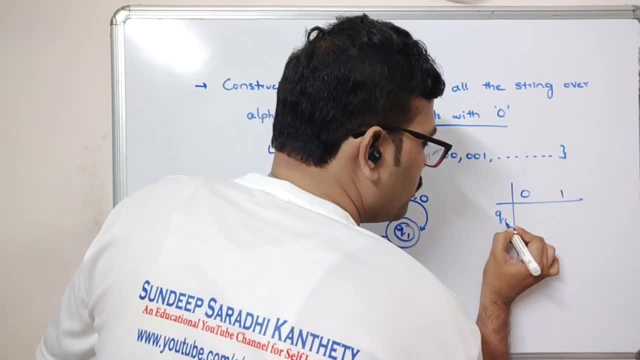 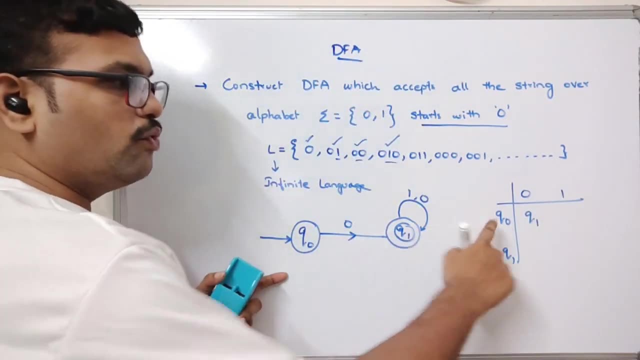 and C. so this is a states q 0 and q 1. so what happens if q 0 with 0? it moves to q 1. what happens if q 0 with 1? so there is no transition here. so it is not a DFA. 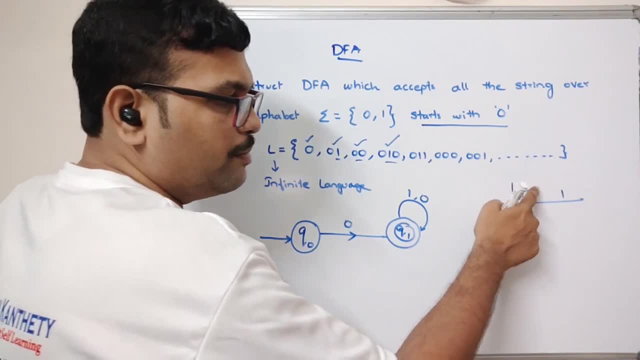 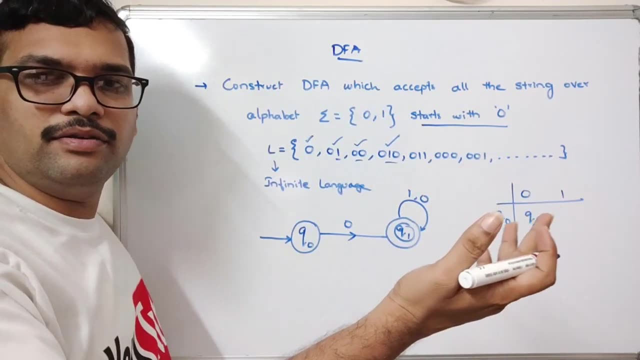 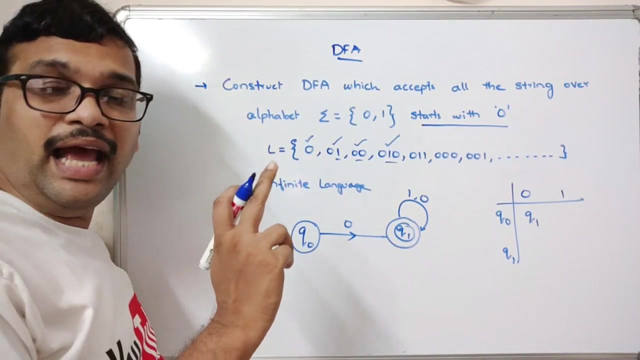 it's not a complete DFA, because for every state, for every input symbol, there should be a transition. okay, let it be. either it can be in the same state or may change it to its state, right, but there should be a transition for every state with a input symbol. only one transition, right, exactly one transition. so we can simply use. if you use, 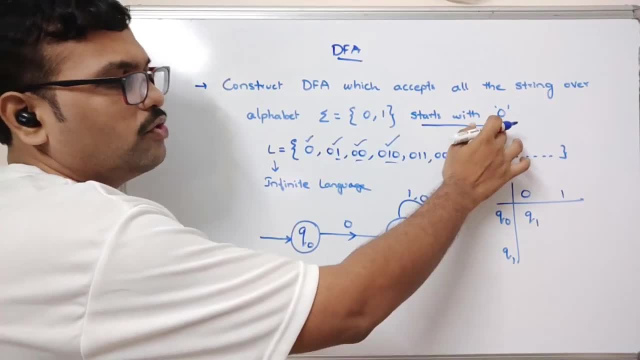 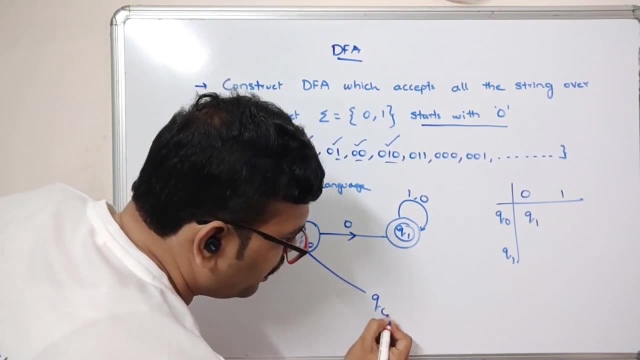 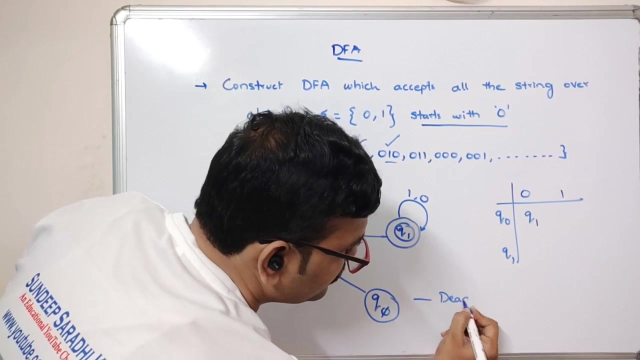 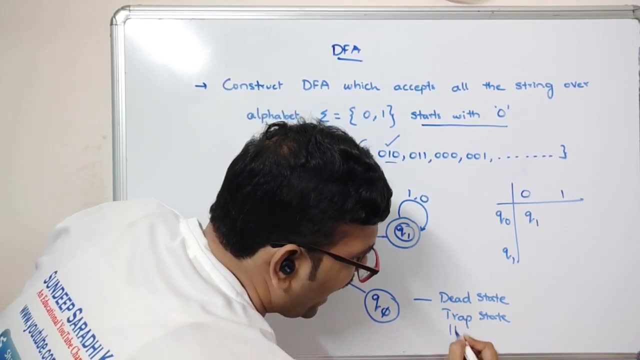 a self loop. if you use a self loop, and here the constraint is starts with zero, so it violates that one. so simply, you can give one state called dead state. you can give the one state called, so this is called dead state, dead state or trap state or hang state. 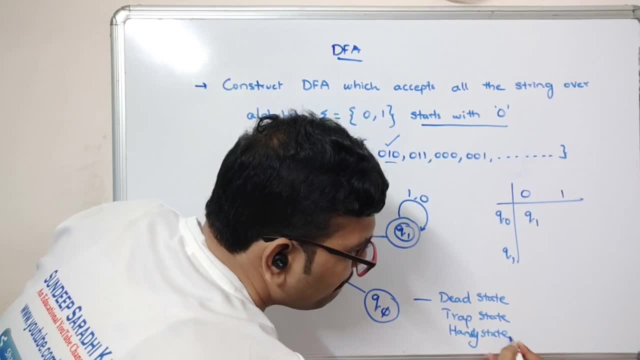 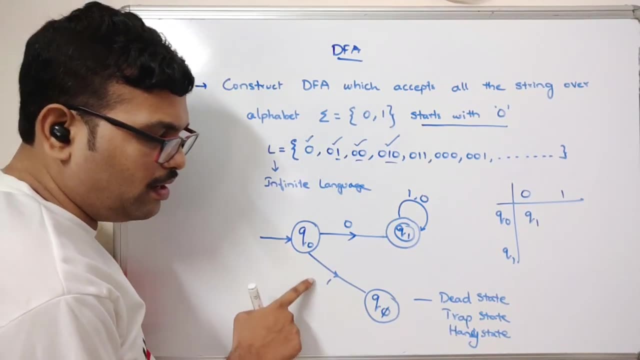 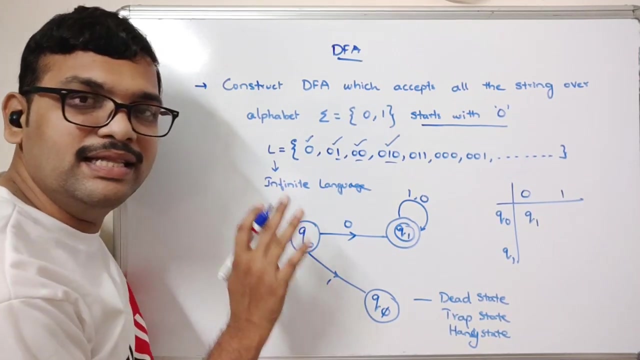 hang state. right. so what is the use of this dead state or hang state or trap state? so whenever the process comes into this state, the process will never go back to any other state. it will remain in this state itself. so whenever you got a q0 with one, it will come to the dead state and it will remains. 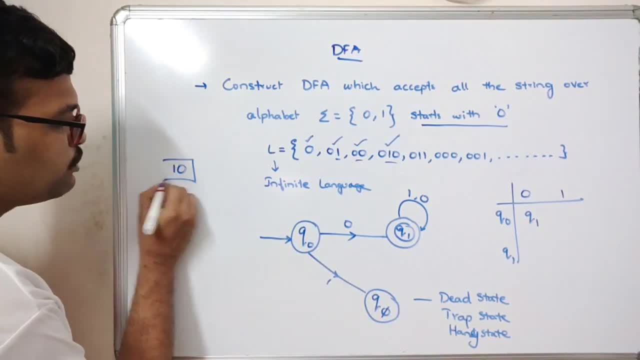 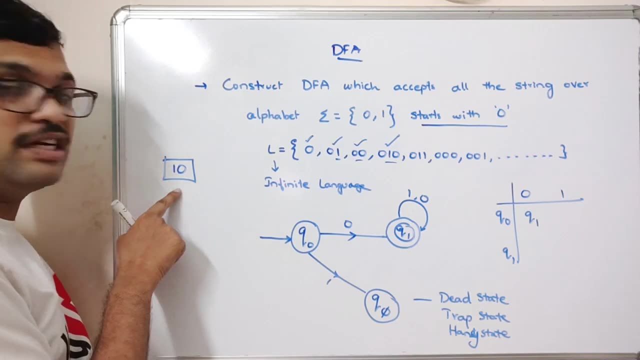 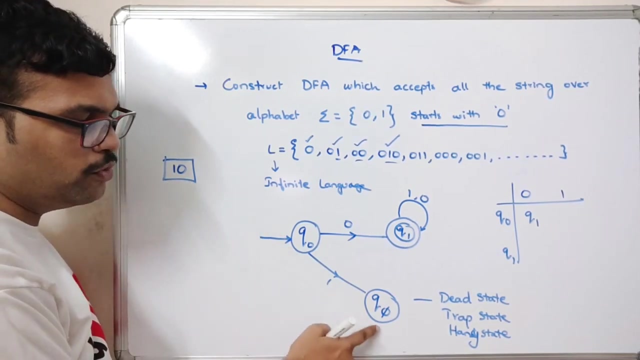 here itself. because if you observe, if you take the string, this one, so this doesn't belongs to this language. so our DFA should not accept this string, because this string doesn't start with zero. so that's why if you get one here, so q0 on one, it moves to the q5, that's a dead. 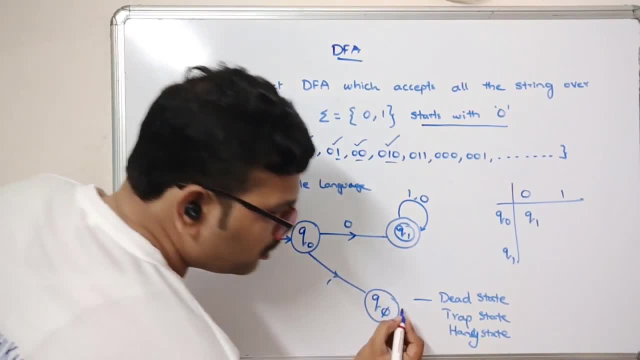 state, so it remains here itself. so here also we can have. so that's why if you get one here, so q0 on one, it moves to the q5, that's a dead state. so here also we can have the transitions zero and one self known, because for every 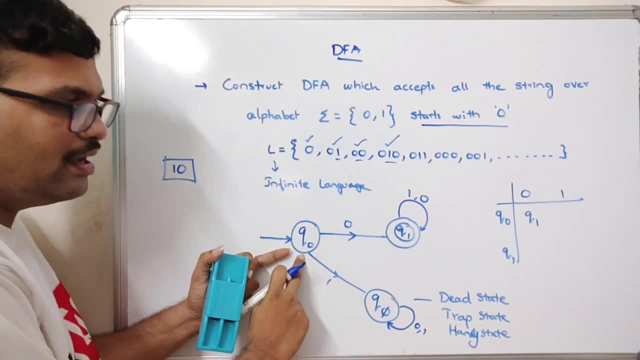 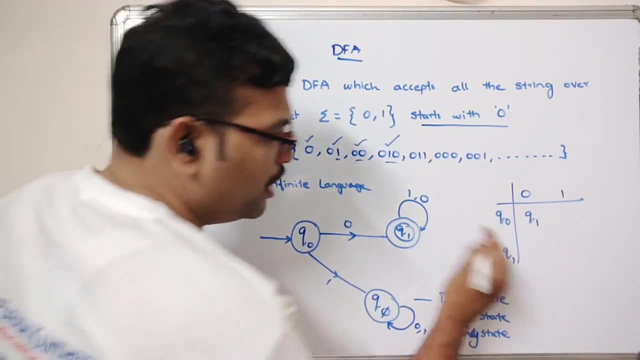 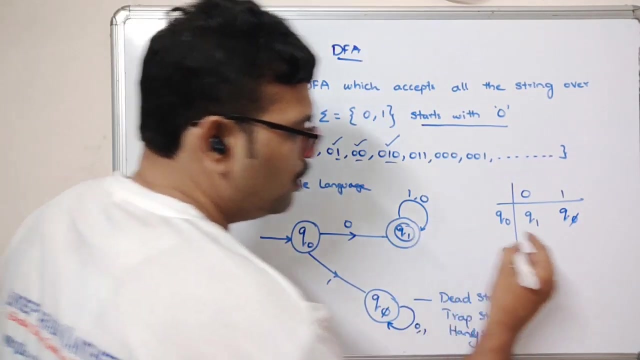 in a DFA. in a DFA for every state, there should be a transition of every symbol. so here we are having q0, q0 on zero, q1. now you can see q0 on one. it goes to q5. this is also a state, but it's a dead state. and what about q1 on zero? it will be in q1 and q1 on one it will. 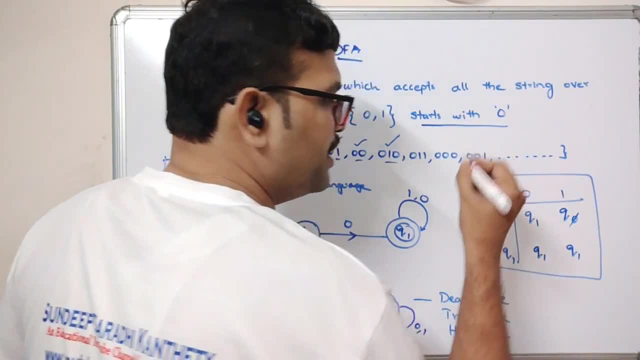 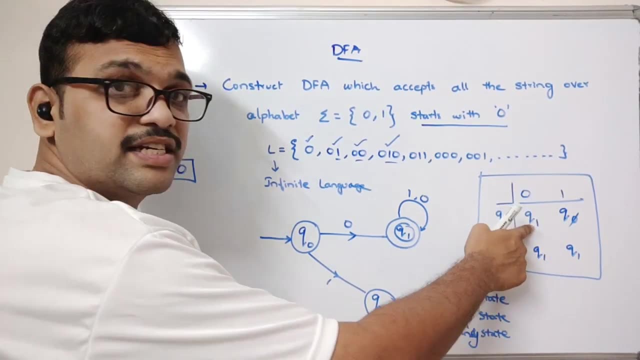 be in the q1, so you can observe here the table is still the same, but it's a dead state, so the table is complete. the table is complete. so for every state there is a transition with a input symbol, so it gives the state. it may remain in the same state or it may change. 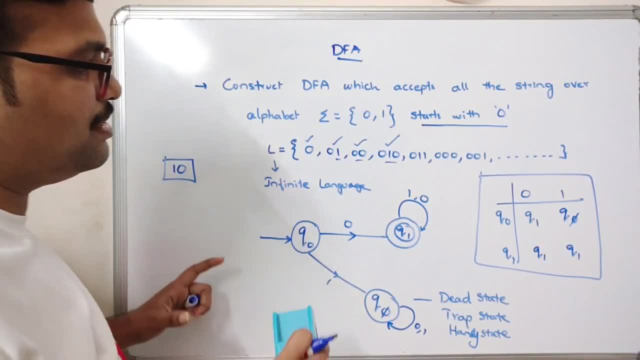 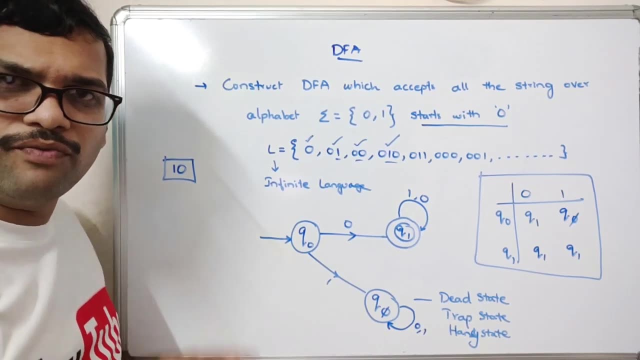 its state right. so this is the construction of DFA for a. start with problem, start with problem. hope you understood this one. one thing you have to remember: for every state in the DFA there should be one transition for every input symbol. so if you are using some q0 on, 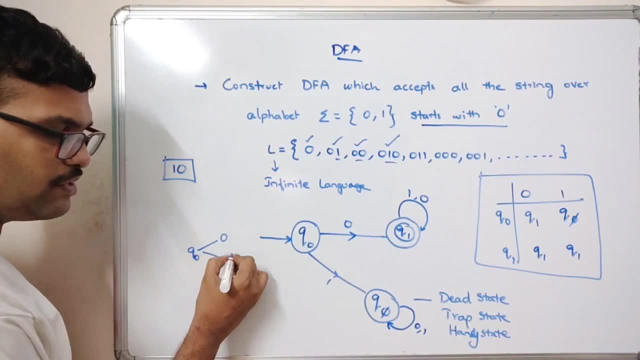 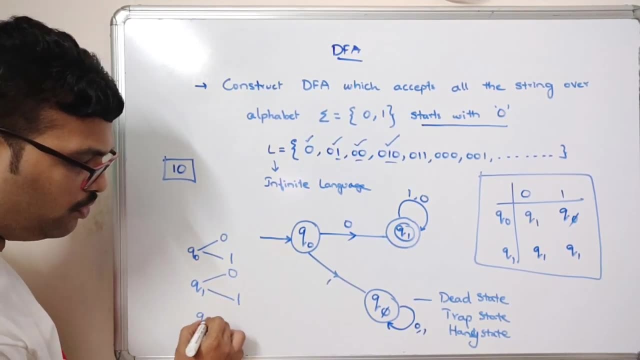 q0, so there should be a transition with zero, there should be a transition with one. and if you are taking q1, there should be a transition with zero and there should be a transition with one. and if you are using q2, there should be a transition with zero and there should. 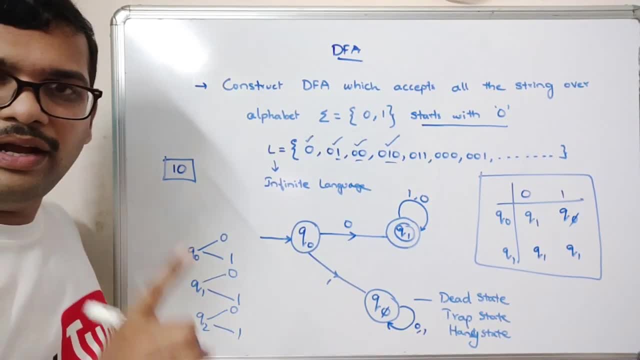 be a transition with one- and this transition also only one, exactly one occurrence- right. so this is called a DFA construction and this is the condition: starts with right. so now we will take one more example and I will construct the DFA. hope you understood this one one thing. 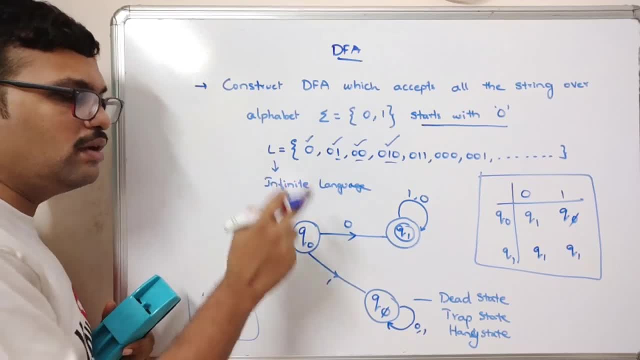 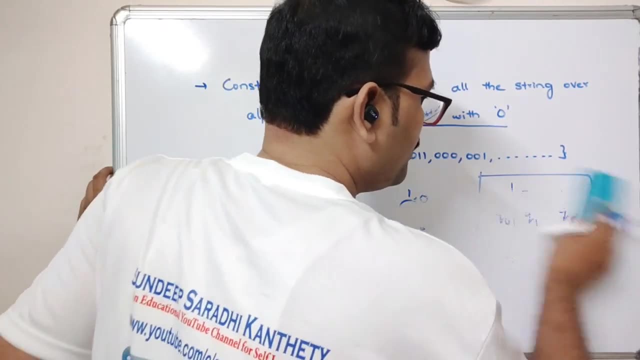 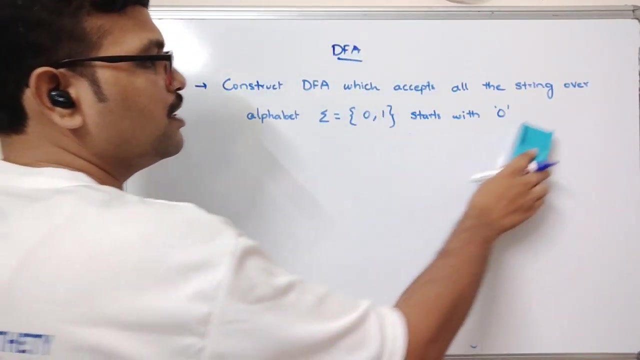 I am going to be. first we need to write the language and then we have to construct the DFA which accept all the strings of this particular language. now let us take one more example, so we will take length: two strings, okay. starts with zero one. stars with zero one. now first, 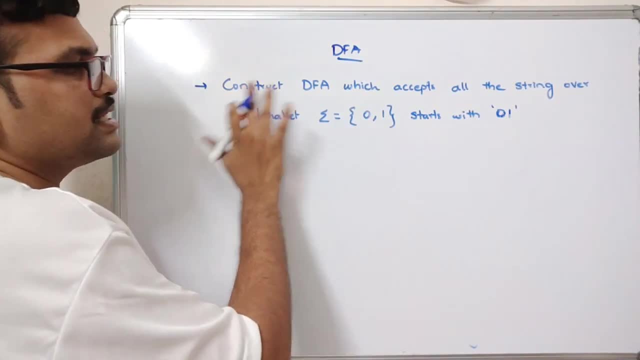 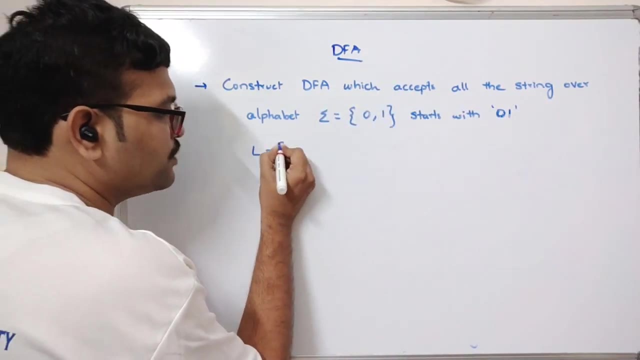 we need to construct the language. see here the construpt, the DFA, which accepts all the string over the alphabet zero one starts with zero one. now, first we need to construct a starts with 01. so construct the language first, write down the language. so what's the minimum? 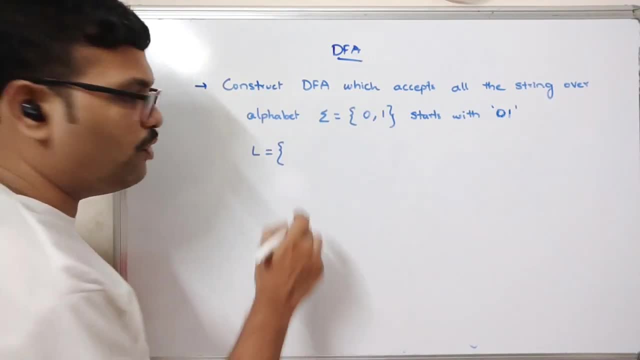 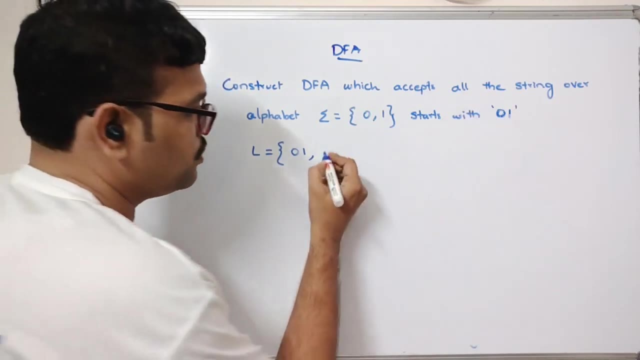 minimum length. so here it is a 2, so starts with 01. so that's why 01 will be the 1, and just after 01 we can have a number of 0s and number of 1s. so that's why i'm taking 010 as a next one. 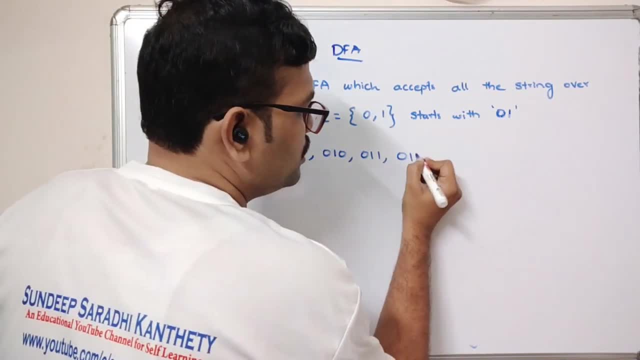 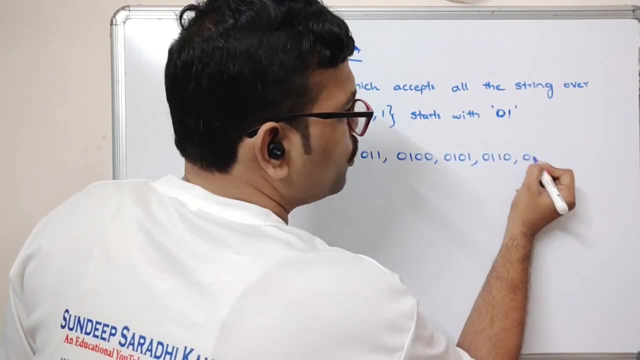 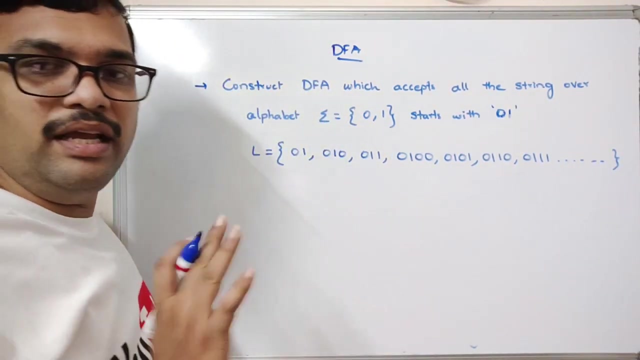 011 as a next one, next 01 00 is a next one, 01 01 is next one, and 01. 10 is next one, 01 11 and so on. so this is also an infinite language. this is also an infinite language, but here we are starting with the minimum and we are going with the maximum. now we have to. 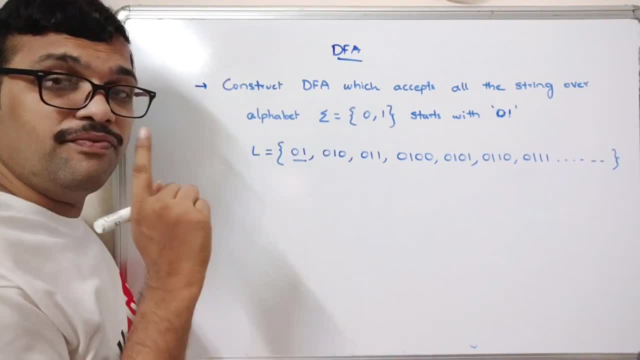 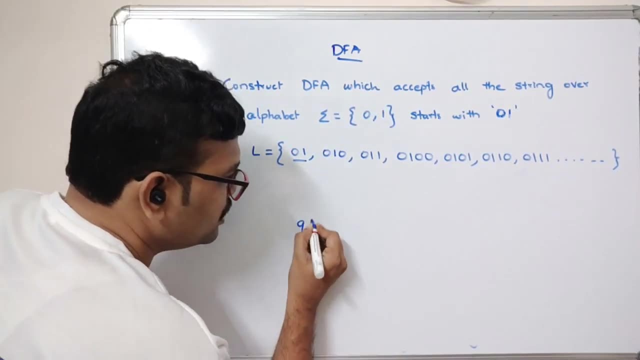 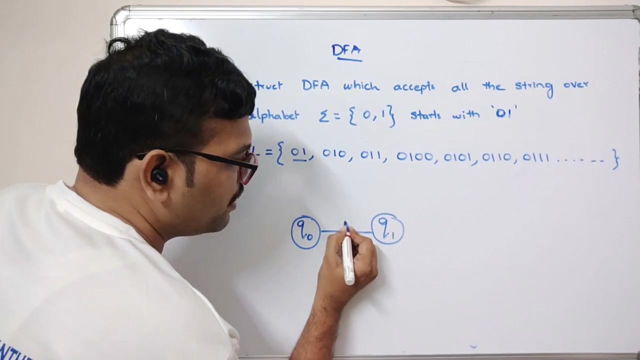 construct this one. what is the minimum string length? 2. so if minimum string length is 2, it requires a three states to construct the dfo. so just write down the this one: q naught q1, see 01. simply write here: 0, q1. 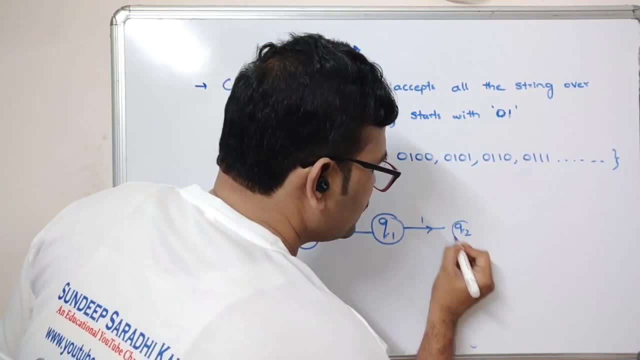 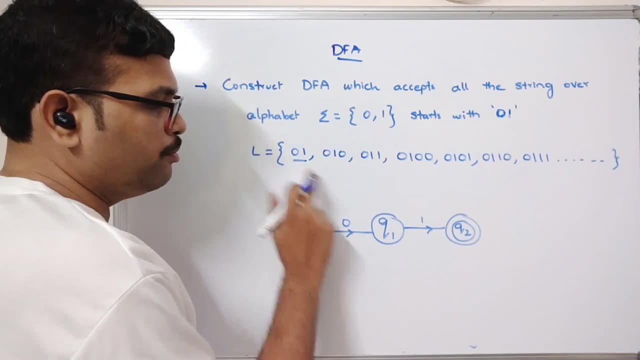 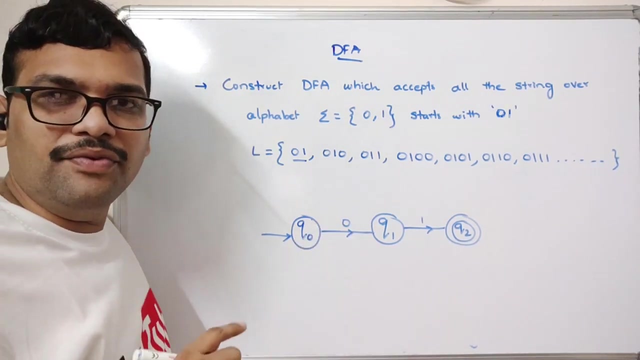 q1, q1 and it goes 1 and it reaches the end state. it reaches the end state, right so? 0, q0 on 0, it moves to q1. q1 on 1, it moves to q2, which is a final state, right so? but this is not a DFA, because 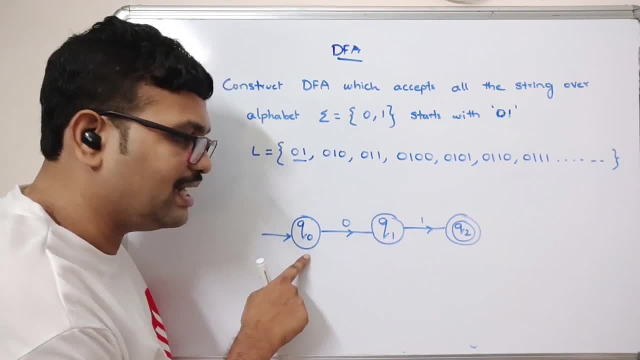 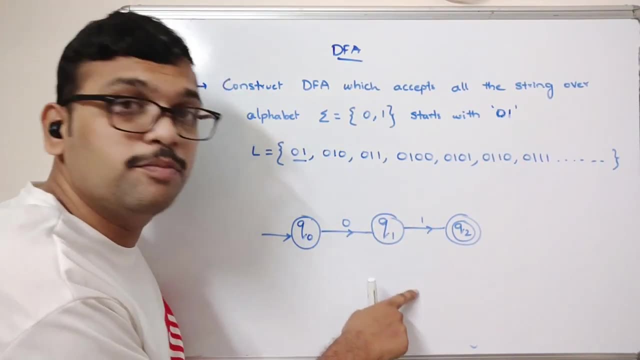 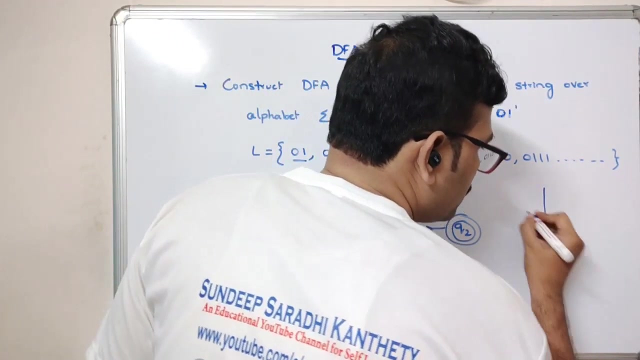 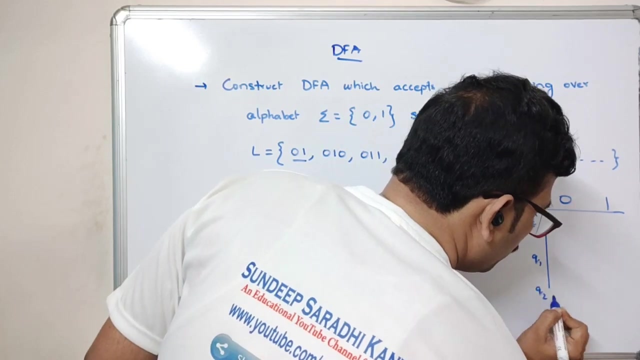 q0 is having a transition for 0, but q0 is doesn't have any transition for 1, and also q1 is having a transition for input symbol 1 and there is no transition for input symbol 0 and q2 doesn't have any transition for input symbol 0 and 1. so here the symbol r, 0, 1 and q0, q1, q2, so q0 on 1, q0 on 0. 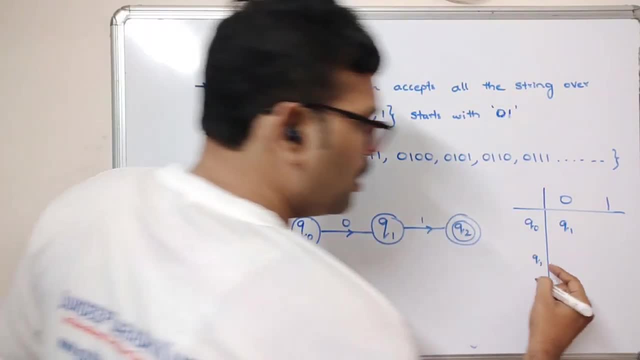 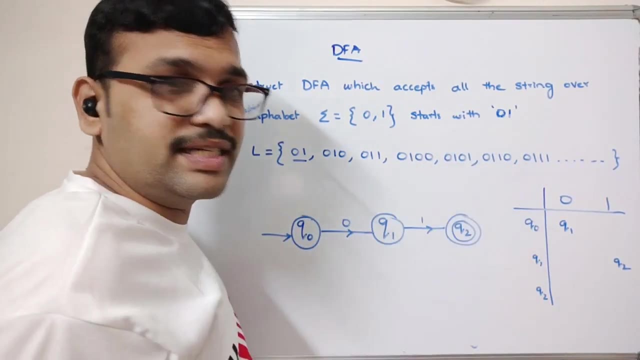 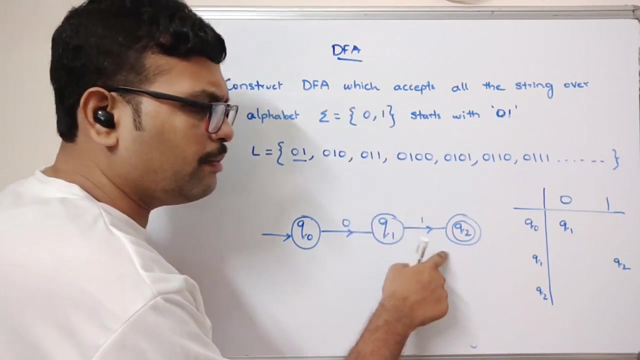 it moves to q1 right and q1 on 1 it moves to q2. what about the remaining? we need to construct such that it should accept all the strings: next 0, 1, 0, 0, 1 and next it is 0. either it may be 0 or 1 it. 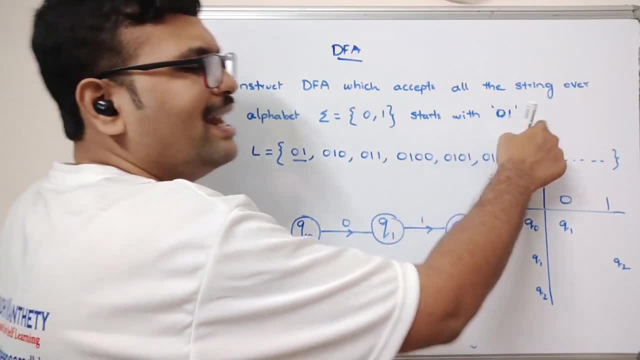 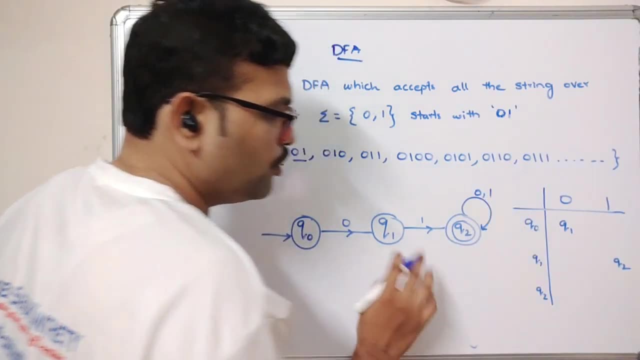 remains in the same state, right, because starts with 0- 1, ending with any number, either 0 or 1, so we can simply use a self loop: 0 or 1, so you can see q0 on 0. it remains in the same state and. 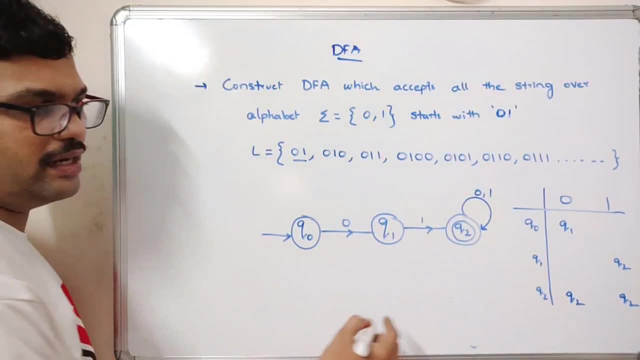 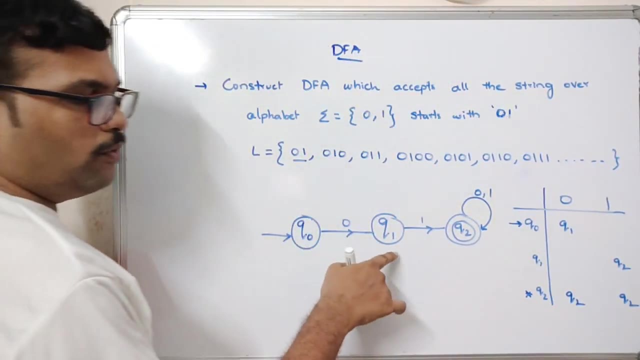 q2 on 1, it remains in the same state. so that's a final state. so you can see here. so this is the initial state and and this is the final state right now. what about the q1? so q1 upon 1, it moves to q2. what about? 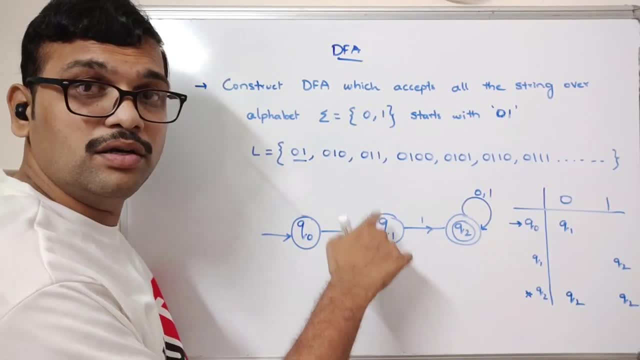 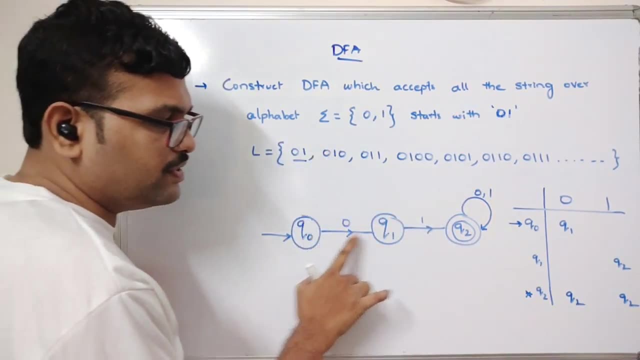 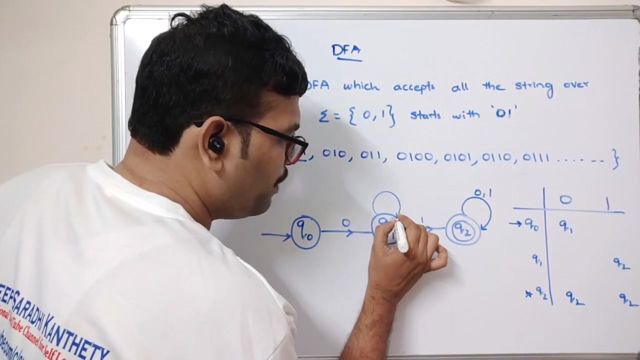 the q1 on 0, q1 on 0. so if it is q1 on 0, automatically it will be violated, because every string should start with 0 and 1. every string should start with 0 and 1. see, for example, if you give a self loop and if you go with the 0. okay, if you go with a self loop and if you 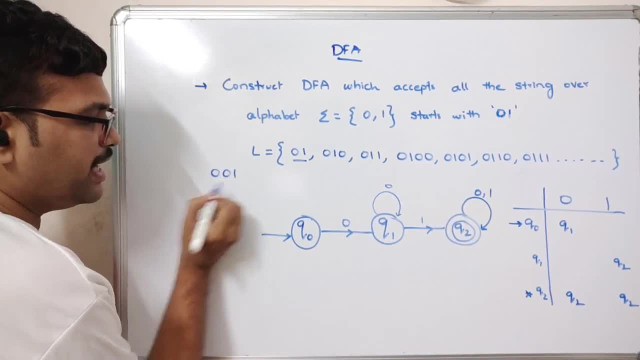 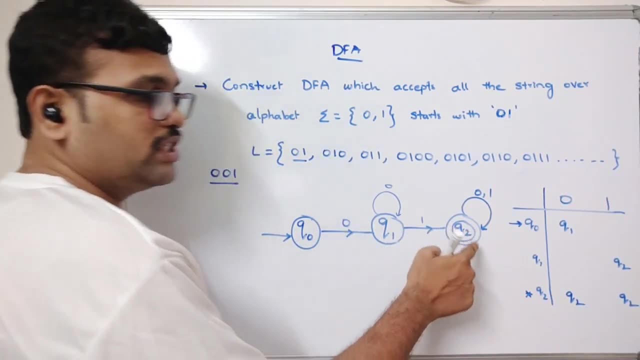 move on with a zero and, if you want, if you are taking the string 0, 0, 1, you can see: q0 on 0 goes to q1, q1 on 0 goes to q1, q1 on 1 goes to q2, which is a final state. so this string is accepted. but 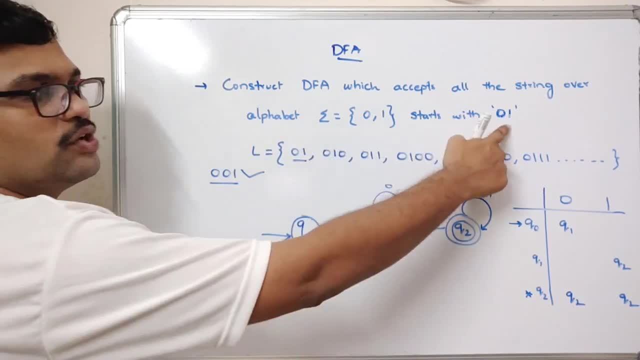 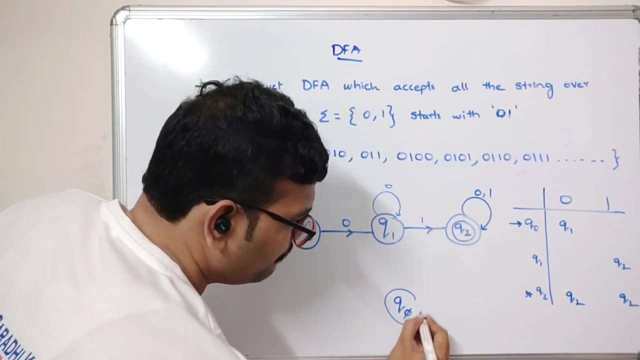 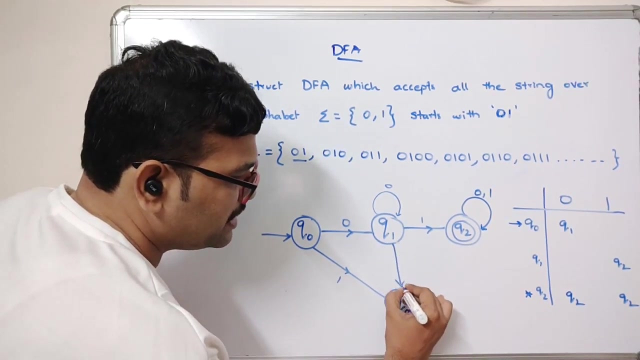 it is not a valid string because it doesn't start with a 0- 1. so that's why just use a dead state and simply pass the transition for 1 to the dead state. so that's why just use a dead state and here also, if it is 0, pass it to the dead state and give the self loop for the dead state. because 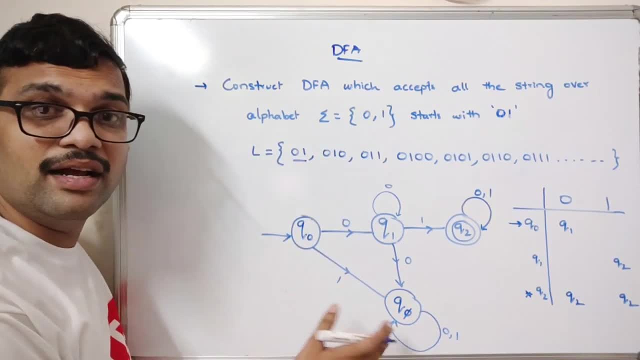 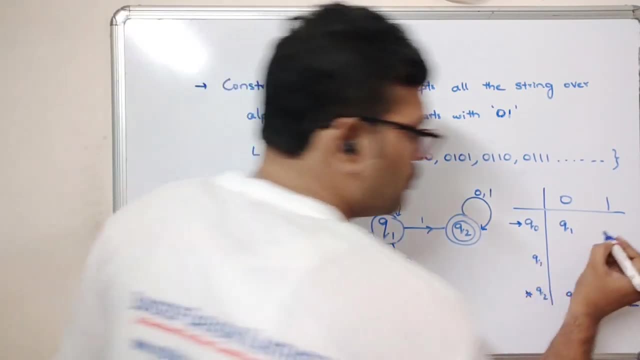 once the process came to the dead state, it will remains in the same state itself. right now you can see q0 on. q0 on 1- it moves to q dash. that's a dead state. and q1 on 0: it moves to q dash. so 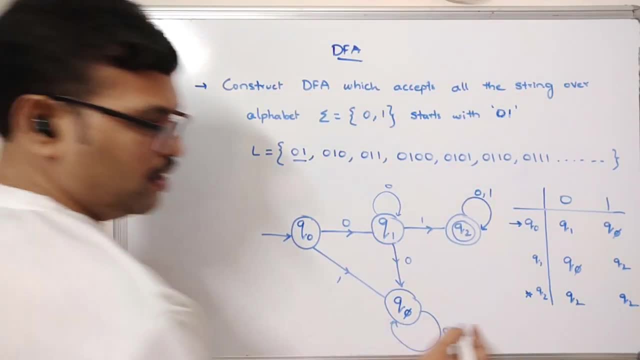 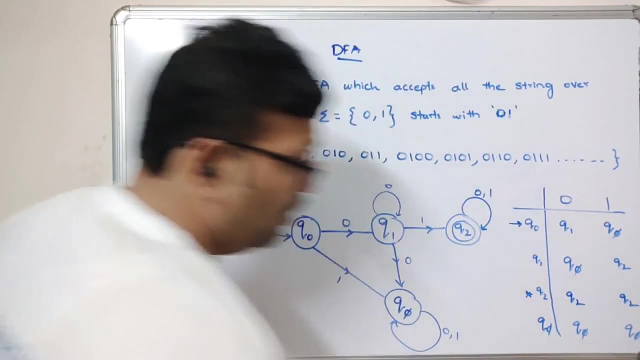 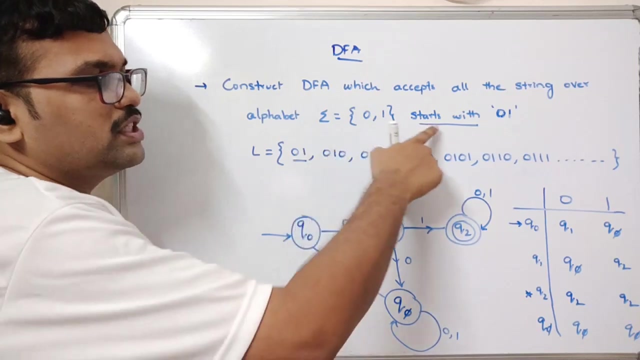 this is also a dead state, right and simply. you can write here: q0, q5, q1 on 0, it moves to q dash, so q5 will be remains in the same state. so in the problems which which is having the starts with problem, so all the dfs which starts with problem will be having this dead state, dead state. 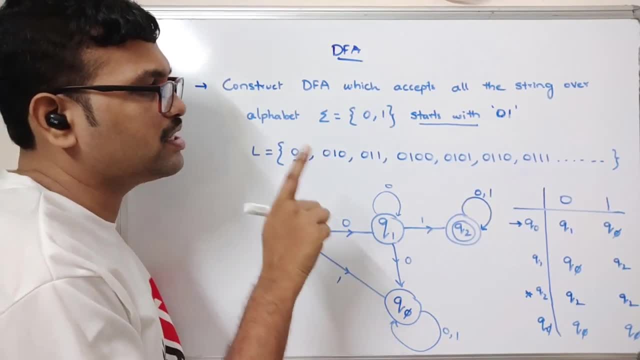 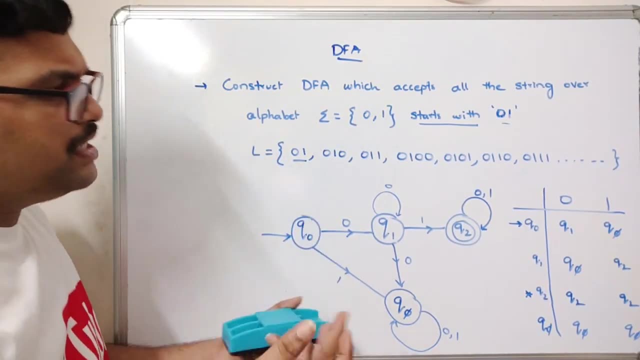 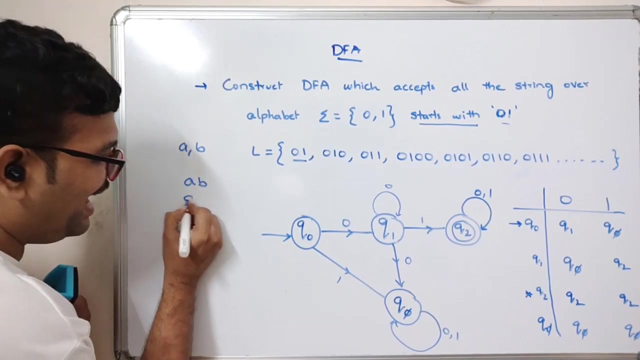 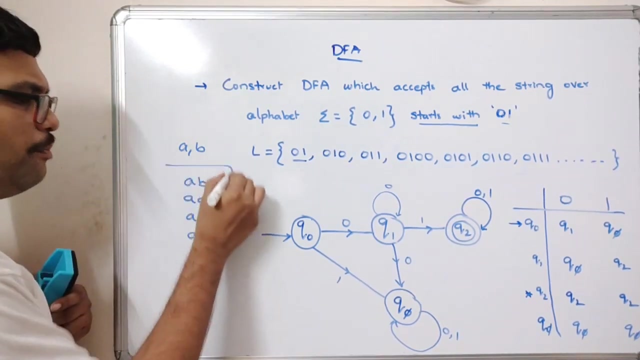 because there is a restriction for that. all the strings should start with 0, 1, right, 0, 1. hope you understood this one. so you might be seeing the input alphabets like a comma, b and there will be a question which starts with a, b or a, a or a, b, a or right, so a, a, b and so on. so these are the. 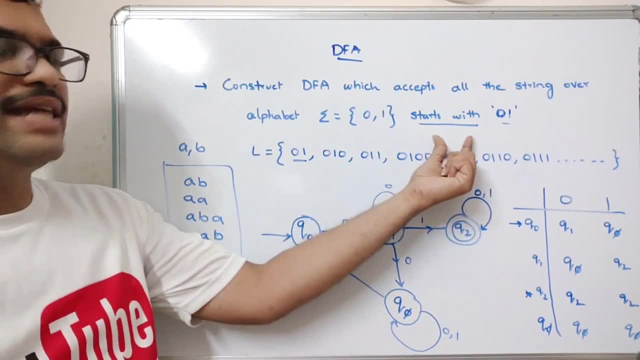 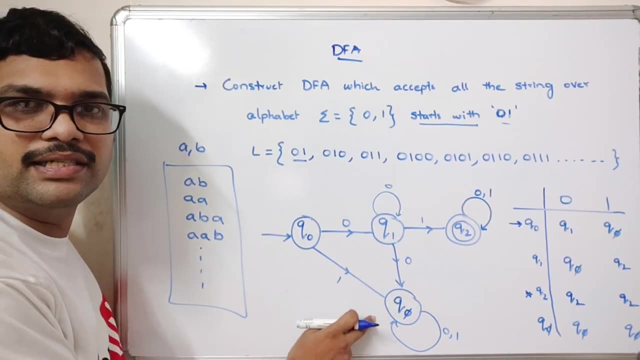 possible problems which can come under this category. that is a starts with, so every time if it is a starts with problem, there will be a dead state. there will be a dead state, and first you need to write the language with all the accepted strings and then you have to construct the dfa. 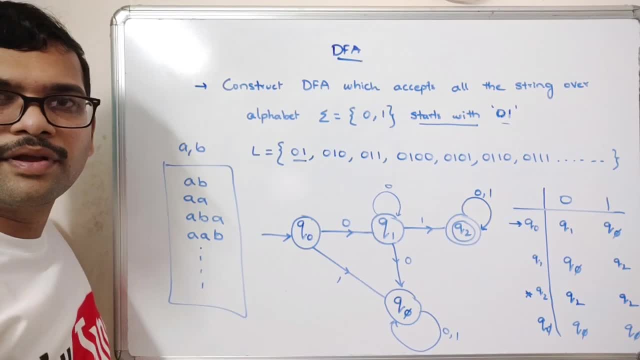 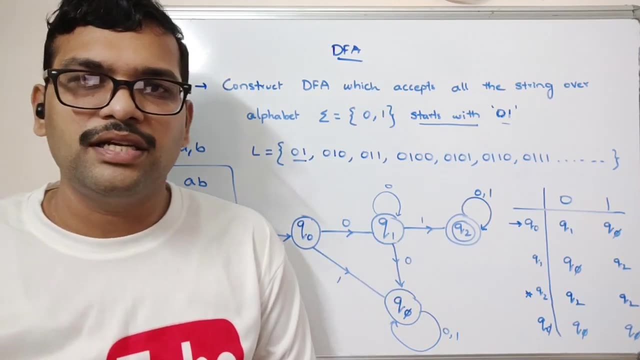 and then you have to write the transition table right. so hope you understood this one. so if you are having any doubts regarding this starts with problem, feel free to post your doubts in the comment section. definitely, i will try to clarify all your doubts and if you really enjoyed my session, like my session, share my session with. 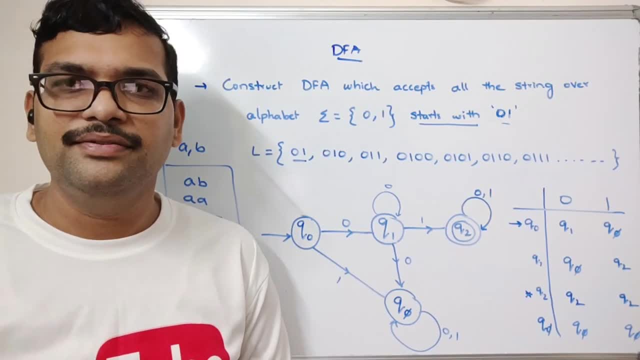 your friends and don't forget to subscribe to our channel. thanks for watching. thank you very much.